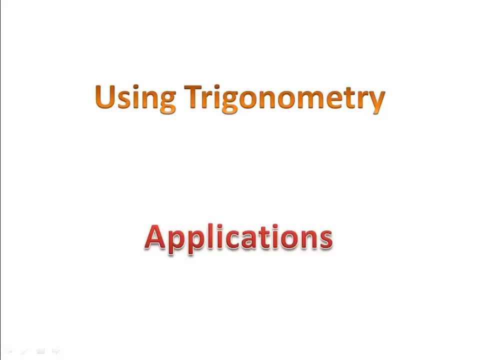 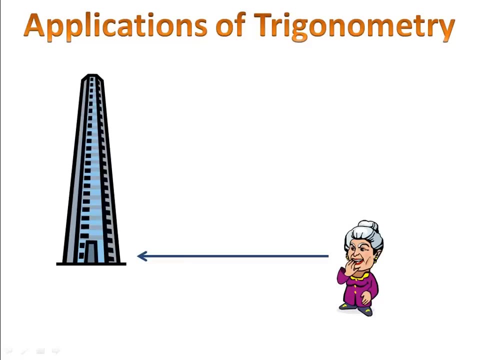 In today's lesson we're going to take a look at some applications of trigonometry. Suppose we have a building, We have a little old lady down on the ground and she's looking at the bottom of the building. She decides to look upward, toward the top, The angle that's been 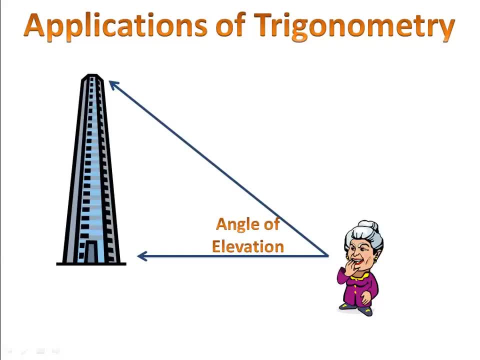 formed by her looking up is called the angle of elevation. You can remember that, because when you look up it's called elevation, and if you want to go up you'll take an elevator. Now suppose the little old lady gets inside the building. she takes the elevator to the 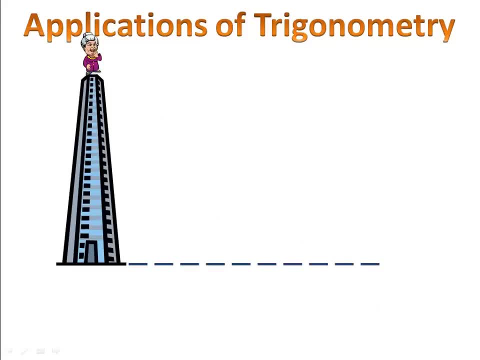 top. and now she's standing up on the top of the building. She's looking straight ahead into the horizon. She decides to look down to the ground. The angle that's formed when she looks down is called the angle of depression. You can remember that, because if you have 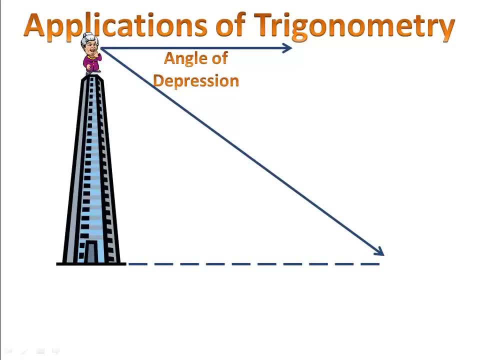 depression, you'll feel down. So what does this really mean? Well, first of all, here's an interesting fact: The angle of depression is always the same as the angle of elevation. So if the angle of depression is 45 degrees, 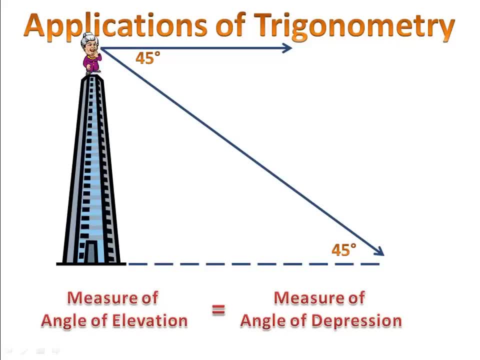 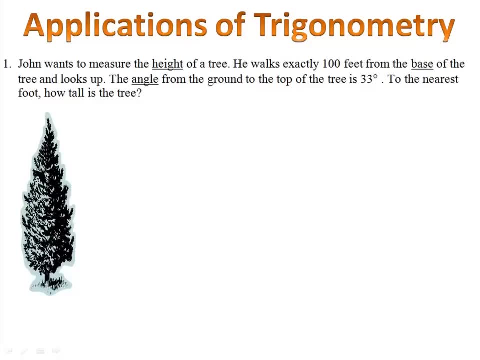 the angle of elevation is also 45 degrees. This is actually very handy, and you'll see how this is as we look through some examples. In example one, we have a tree. John wants to know how high the tree is, but he doesn't. 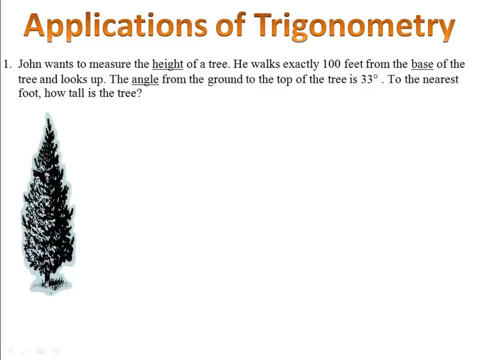 really feel like climbing up to the top and measuring down. He decides to use trigonometry. Whenever we use trigonometry, we're talking about triangles, and so we'll draw a triangle next to the tree. He walks 100 feet from the bottom of the tree, and so we'll begin by labeling. 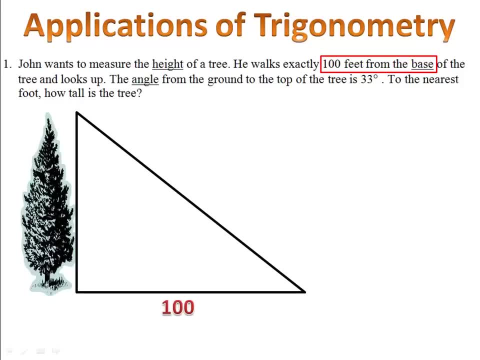 our triangle: 100 on the bottom. That's the side, that's on the ground. Then he looks up: The angle of elevation is 33 degrees, and so we'll label that in our triangle also. Now the question says how tall is the tree? Well, you can see that the tree is about 45. 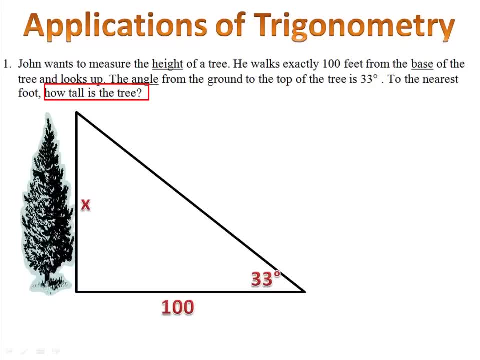 That's what I want to find out, and so I'll call the side along the tree x. Notice that I have here the opposite and the adjacent. Which of our three trig ratios uses the opposite and the adjacent? Well, that's the tangent. 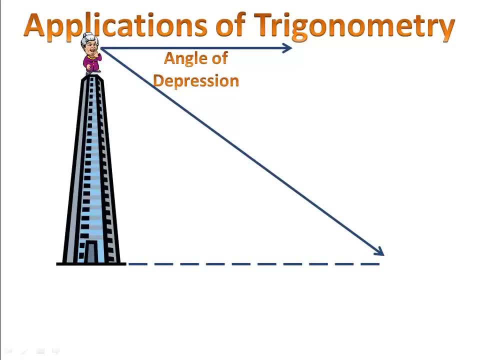 depression, you'll feel down. So what does this really mean? Well, first of all, here's an interesting fact: The angle of depression is always the same as the angle of elevation. So if the angle of depression is 45 degrees, 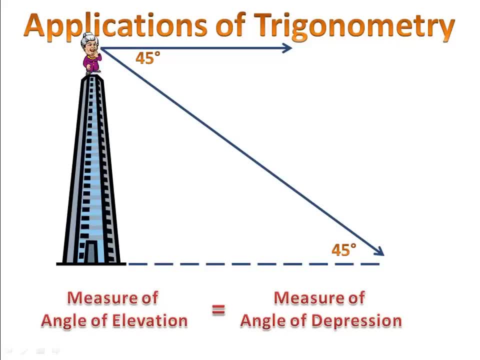 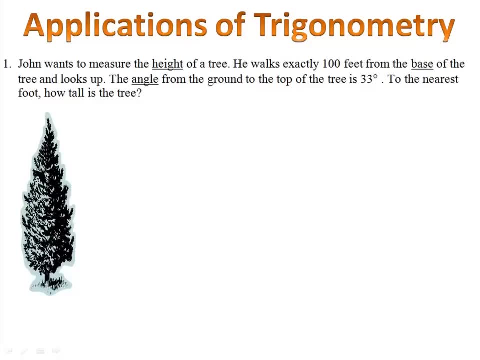 the angle of elevation is also 45 degrees. This is actually very handy, and you'll see how this is as we look through some examples. In example one, we have a tree. John wants to know how high the tree is, but he doesn't. 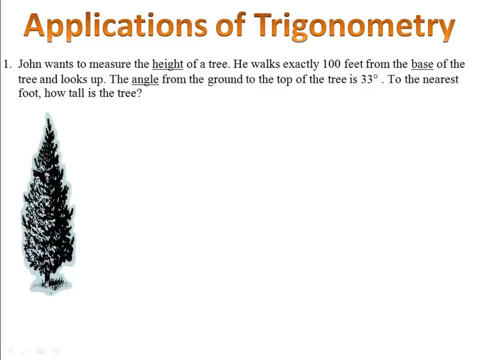 really feel like climbing up to the top and measuring down. He decides to use trigonometry. Whenever we use trigonometry, we are talking about triangles, and so will draw a triangle next to the tree. He walks 100 feet from the bottom of the tree, and so we will begin labeling. 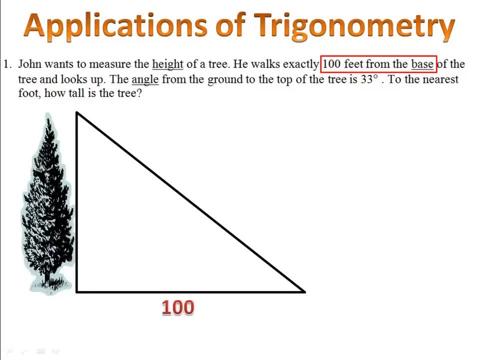 our triangle, 100 on the bottom. that's the side, that's on the ground. Then he looks up: The angle of elevation is 33 degrees and so will label that in our triangle also. Now the question says how tall is the tree, If he's going to talk about the base up and down. 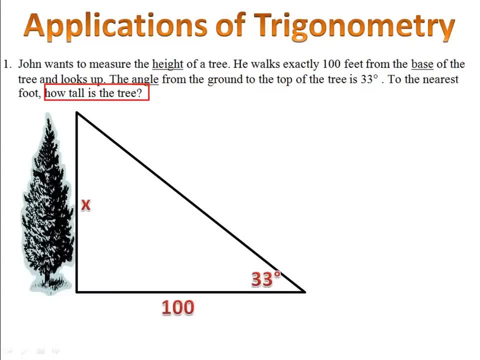 then we'll go with showing him 100 by the height. He says he will first state the height by, and then he will detect if he's walkinguppole, and then he he goes to 100 by the height of the tree. all is the tree. That's what I want to find out, and so I'll call the side along the tree. 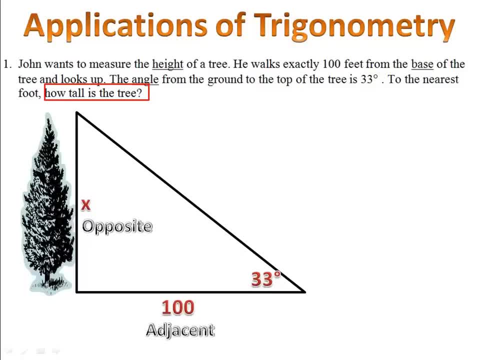 x. Notice that I have here the opposite and the adjacent. Which of our three trig ratios uses the opposite and the adjacent? Well, that's the tangent. So the tangent of 33 degrees equals opposite x over adjacent 100.. Now I can cross, multiply and plug that into my calculator. 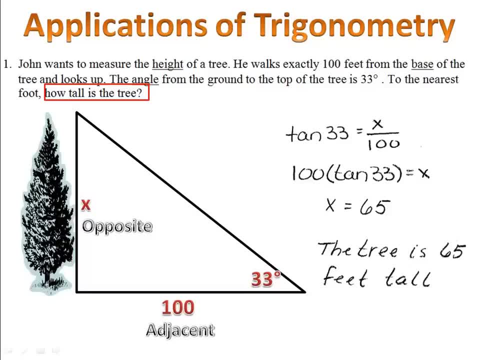 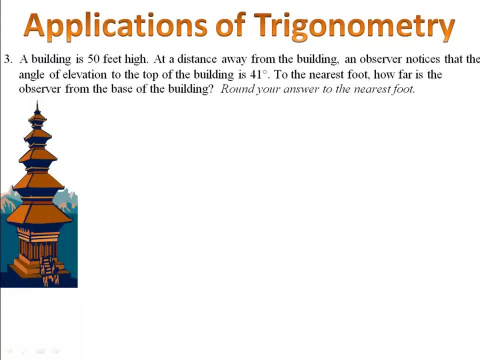 and I get: x equals 65. The tree must be 65 feet tall. In example 3 we have a building that's 50 feet high. We have an observer and he knows that the angle of elevation looking up from the ground to the top of the building is 41 degrees. The question is, how far away? 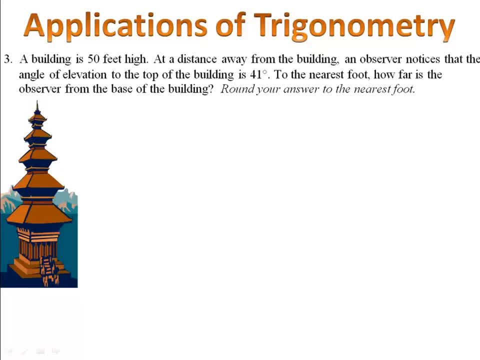 from the base of the building is the observer. Well, we're going to use trigonometry, and so we'll draw a triangle right alongside the building. Now. Now, let's fill in the information that we have. The building is 50 feet high, the angle of elevation is 41 degrees and the observer 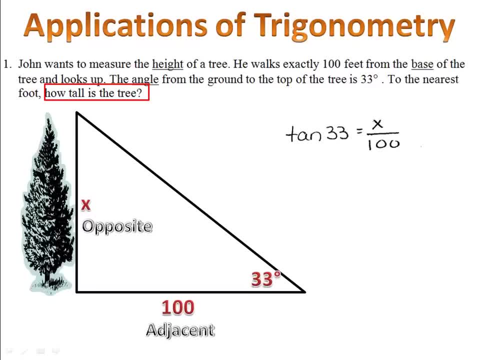 So the tangent of 33 degrees equals opposite x over adjacent 100.. Now I can cross, multiply and plug that into my calculator and I get x equals 65.. The tree must be 65 feet tall. In example 3 we have a building that's 50 feet high. 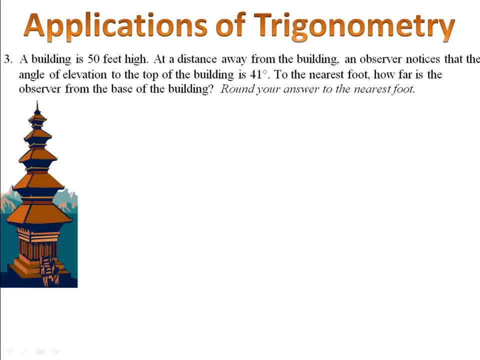 We have an observer and he knows that the angle of elevation looking up from the ground to the top of the building is 41 degrees. The question is: how far away from the base of the building is the observer? Well, we're going to use trigonometry. 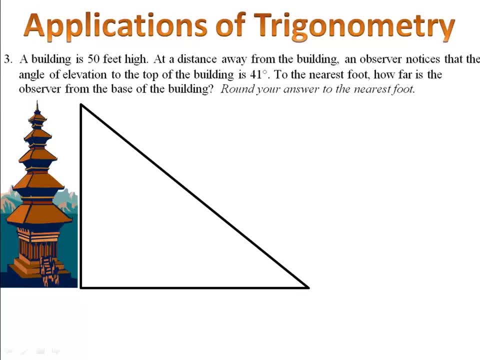 And so we'll draw a triangle right alongside the building. Now let's fill in the information that we have. The building is 50 feet high, The angle of elevation is 41 degrees, And the observer wants to know how far we are from the base of the building. 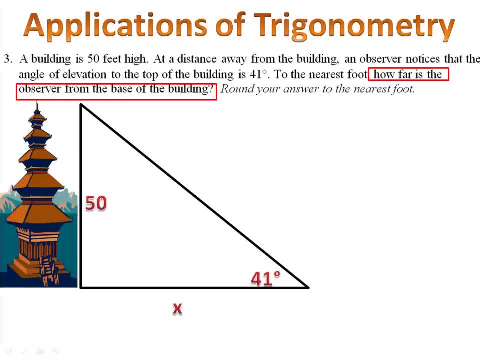 Now that we've filled in our triangle, we can use trigonometry to find the length of that side. Please pause the video here, Find the length of the side marked x And then come on back and we'll see how you did. 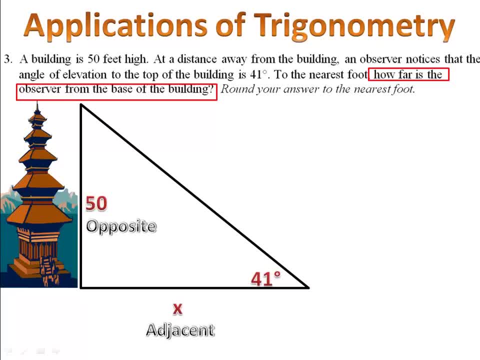 We began by looking at the sides that we have. We had our opposite and our adjacent, Opposite and adjacent is the tangent ratio, And so we have the tangent of 41 degrees equals 50 over x. Now we cross, multiply and solve for x. 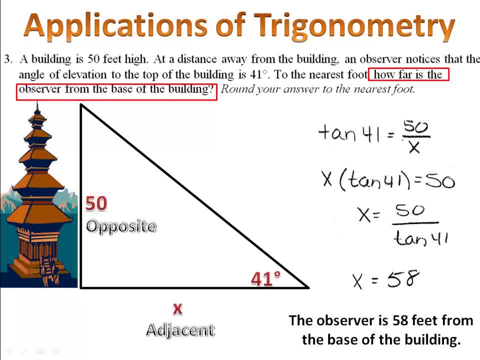 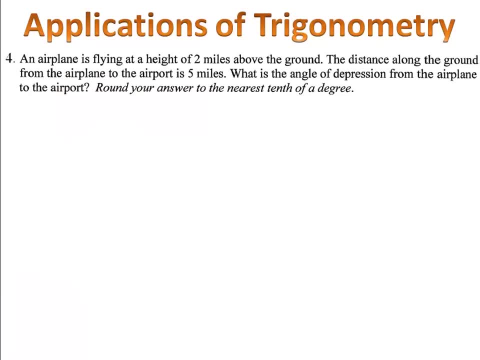 X equals 58,, which means the observer must be 58 feet from the base of the building. Next, let's take a look at example 4.. We have an airplane that's flying at a height of 2 miles above the ground. 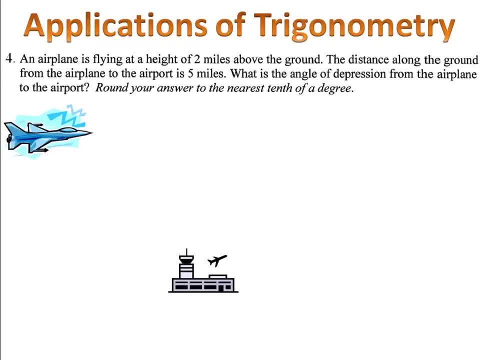 And we know that if we go down to the ground it's about 5 miles from the airplane to the airport. We want to know what the angle of depression is from the airplane to the airport. For example, what angle does the pilot need to put the plane down so that it can land? 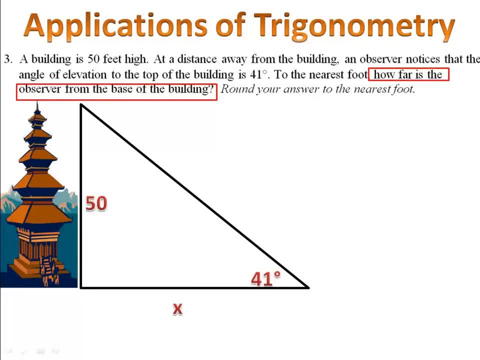 wants to know how far we are from the base of the building. Now that we've filled in our triangle, we can use trigonometry to find the length of that side. Please pause the video here. find the length of the side marked X and then come on back. 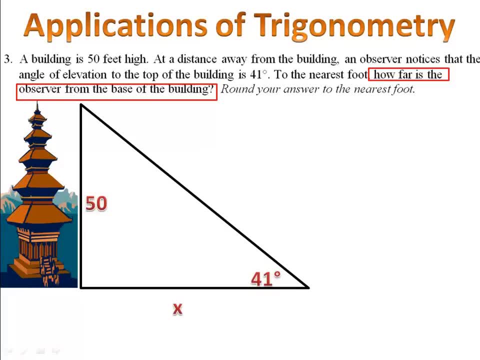 and we'll see how you did. We began by looking at the sides that we have. We had our opposite and our adjacent. Opposite and adjacent is the tangent ratio, and so we have the tangent of 41 degrees equals 50 over X. Now we cross, multiply and solve for X. X equals 58, which means the observer. 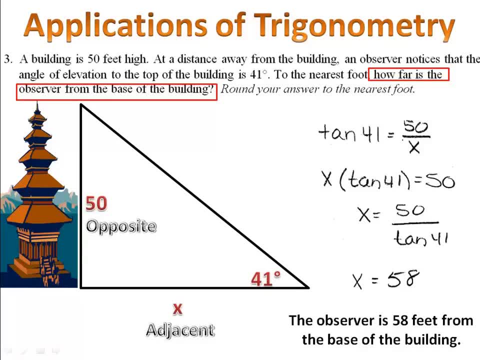 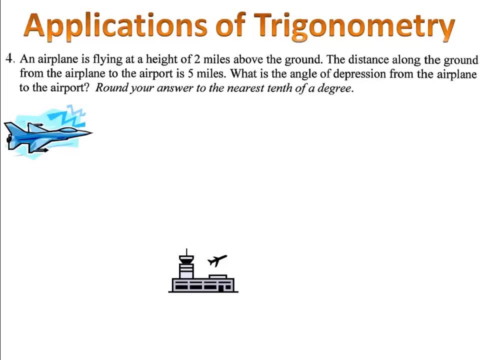 must be 58 feet from the base of the building. Next, let's take a look at example four. We have an airplane that's flying at a height of two miles above the ground and we know that if we go down to the ground it's about five miles from the airplane to the airport. 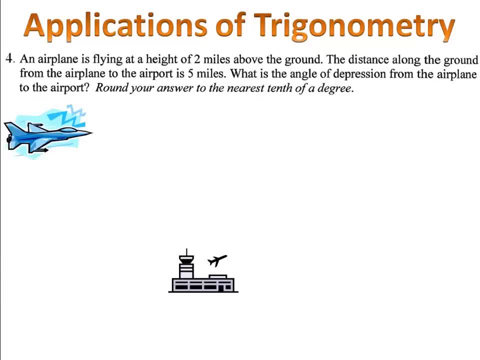 We want to know what the angle of depression is from the airplane to the airport. For example, what angle does the pilot need to put the plane down so that it can land at the airport? We draw a triangle and we label what we have. 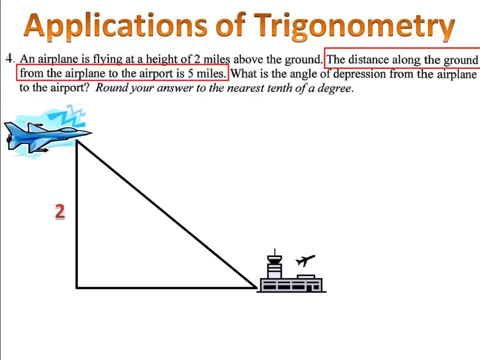 The airplane is two miles above the ground. The distance from the airport to the airplane along the ground is five miles. We want to know the angle of depression, the angle that the pilot's looking down to see the airport. Remember, the angle of depression has the same measure as the angle of elevation. 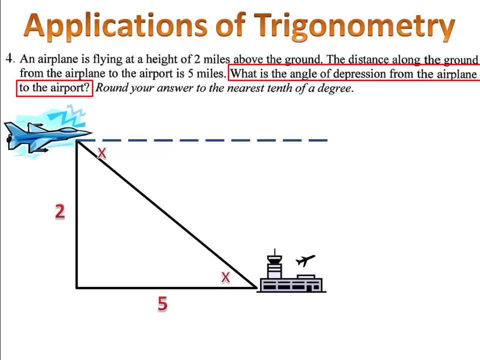 That actually makes sense, because if the pilot is looking down at the airport and the person at the airport is looking up at the sky, Looking up at the airplane, they must be looking at the same angle. Now we can use our trigonometry. 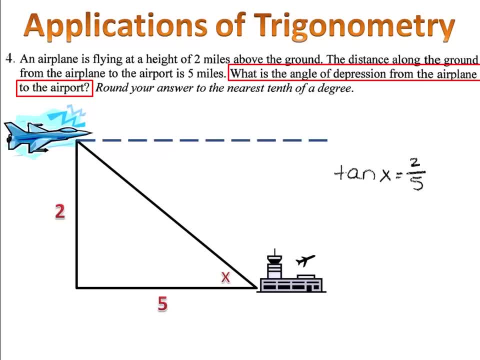 We have our opposite and our adjacent once again. So the tangent of angle x is two over five. Now we find the angle with the inverse and we find out that the angle of elevation is twenty-one point eight degrees, which means the angle of depression is also twenty-one. 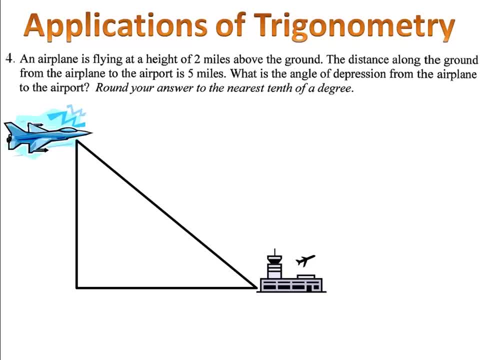 at the airport We draw a triangle And we label what we have. The airplane is 2 miles above the ground. The distance from the airport to the airplane along the ground is 5 miles. We want to know the angle of depression, the angle that the pilot's looking down to see. 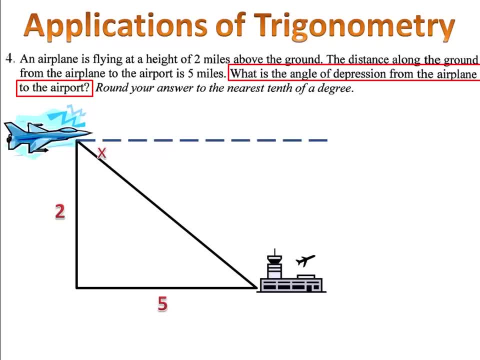 the airport. Remember, the angle of depression has the same measure as the angle of elevation. That actually makes sense, because if the pilot is looking down at the airport and the person at the airport is looking up at the airplane, they must be looking at the same angle. 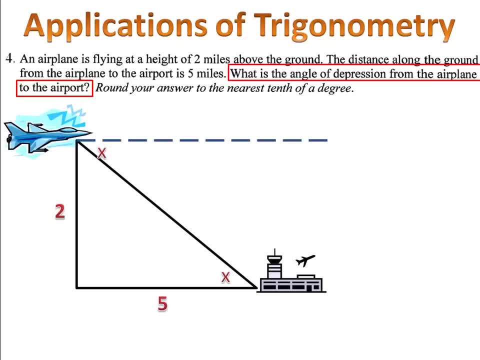 Now we can use our trigonometry. We have our opposite and our adjacent once again. So the tangent of angle x is 2 over 5.. Now we find the angle with the inverse and we find out that the angle of elevation is 21.8 degrees. 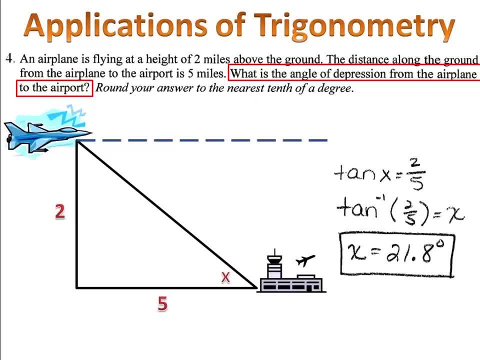 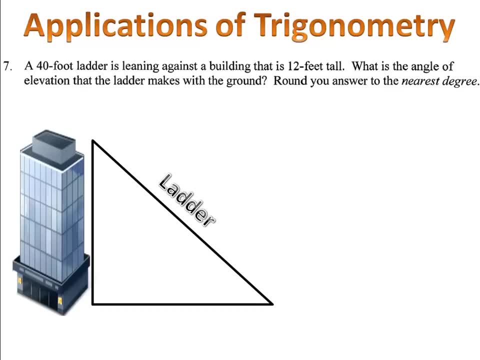 Which means the angle of depression is also 21.8 degrees. Well, that's about it, degrees. Our final example- example 7, is for you to try. We have a 40 foot ladder and it's leaning against a 12 foot tall building. 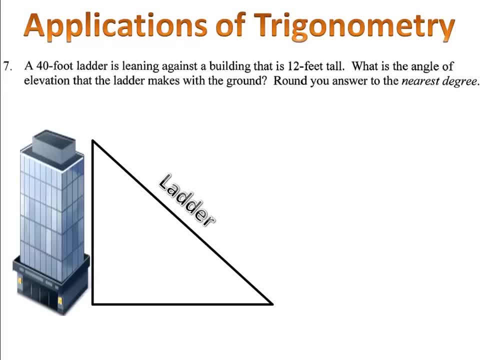 They want to know the angle of elevation that the ladder makes with the ground. Please label the triangle with the sides and the missing angle and then come back and we'll take a look at your work. We began by drawing a triangle. the ladder is the hypotenuse and the left hand side. 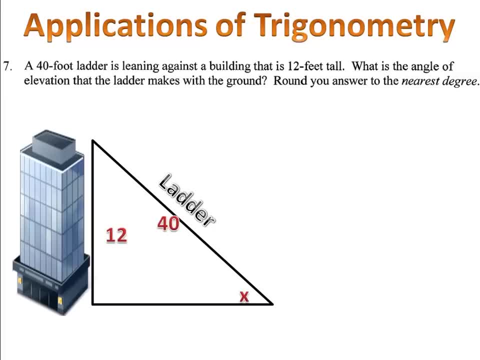 of the triangle is the building. We know that the building is 12 feet tall, the ladder is 40, and the angle of elevation is x. that's what we want to find. Now let's find the measure of the angle. Please pause the video here. find the measure of angle x and then come on back. 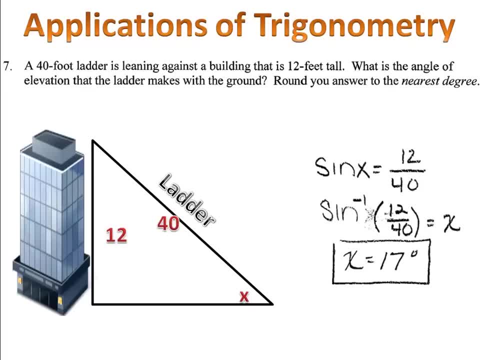 Let's see how you did. We have the opposite and the hypotenuse Opposite, and hypotenuse is our sign ratio. so the sign of angle x is 12 over 40. We use the inverse to find the measure of the angle. 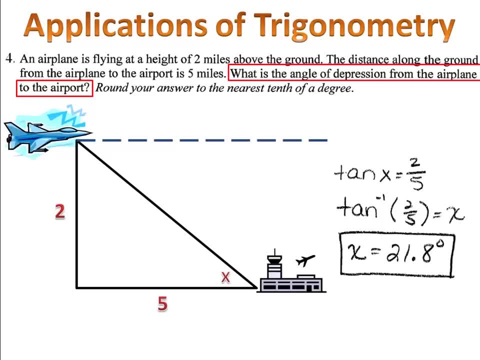 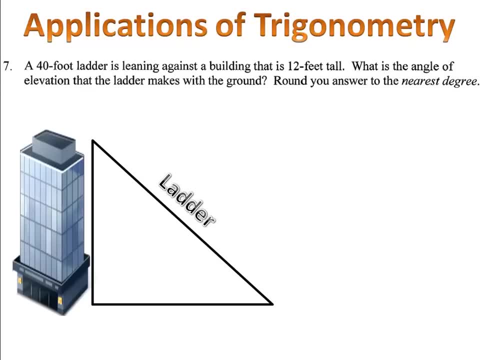 point eight degrees. Our final example, example seven, is for you to try. We have a forty foot ladder and it's leaning against a twelve foot tall building. They want to know the angle of elevation that the ladder makes with the ground. Please label the triangle with the sides and the missing angle and then come back and we'll. 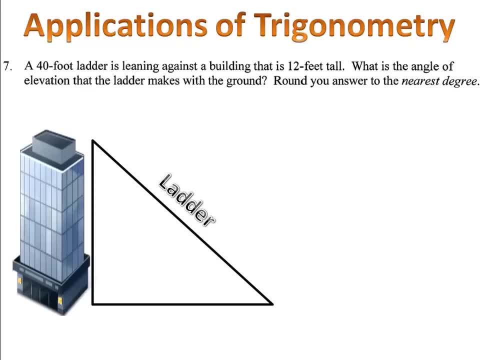 take a look at your work. We began by drawing a triangle. The ladder is the hypotenuse. We're going to draw a triangle. The left hand side of the triangle is the building. We know that. the building is twelve feet tall, the ladder is forty and the angle of elevation 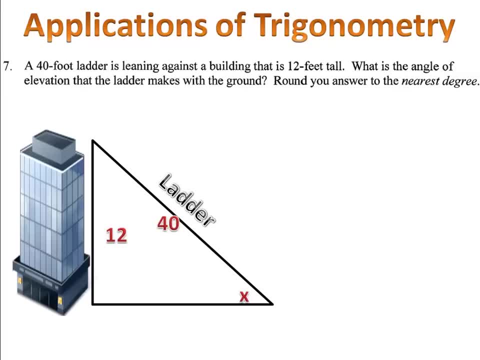 is x. That's what we want to find. Now let's find the measure of the angle- Please pause the video here- find the measure of angle x and then come on back Let's see how you did. We have the opposite and the hypotenuse. 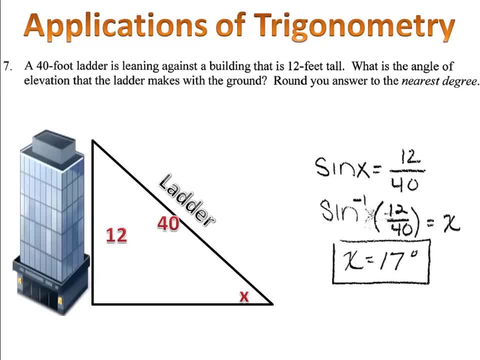 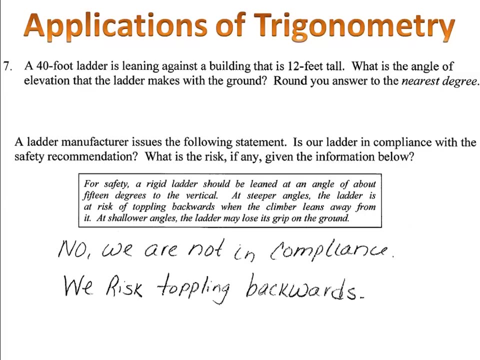 Opposite and hypotenuse is our sine ratio. So the sine of angle x is twelve over forty. We use the inverse to find the measure of the angle. We get that the angle is approximately seventeen degrees. Now, to follow up with this, the ladder manufacturer has issued a statement in the owner's manual. 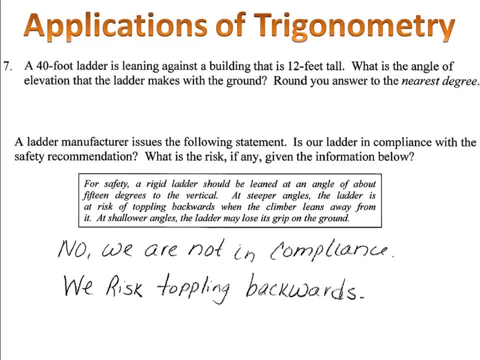 That statement says for safety, a rigid ladder should be leaned at an angle of about fifteen degrees to the vertical. At steeper angles the ladder is going to be leaning at an angle of about fifteen degrees. At steeper angles the ladder is at risk of toppling backwards when the climber leans. 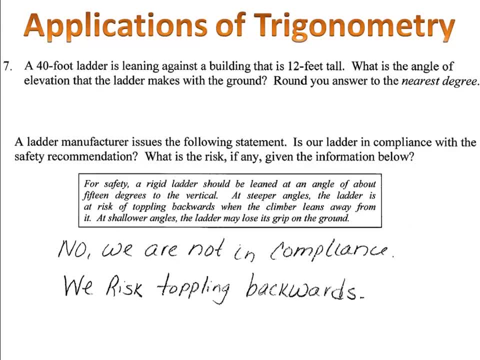 away from it. At shallower angles, the ladder may lose its grip on the ground and fall. Is our ladder in compliance? Well, it says that we should have an angle of no more than fifteen degrees. Our angle happens to be seventeen degrees, which is a problem. 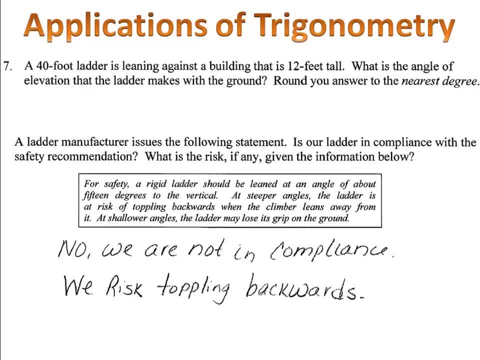 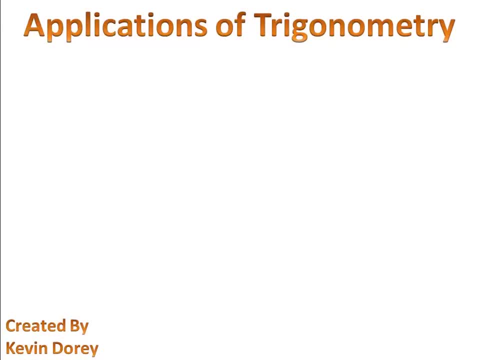 And therefore we're not in compliance. we run the risk of toppling over. So here's everything you need to know About applications of trigonometry. When you have it, draw a picture. Draw a picture of the tree, draw a picture of the building. draw a picture of the lamp.